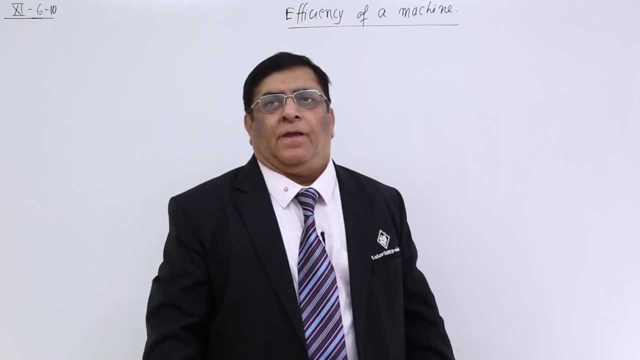 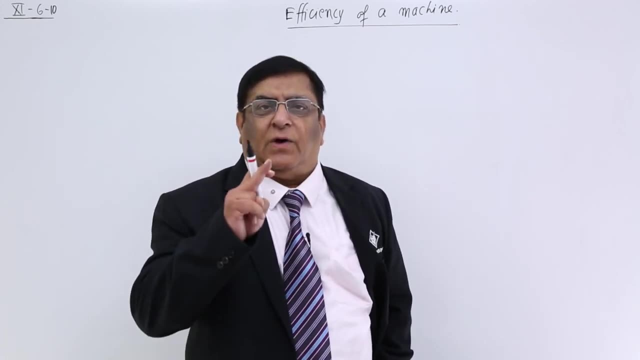 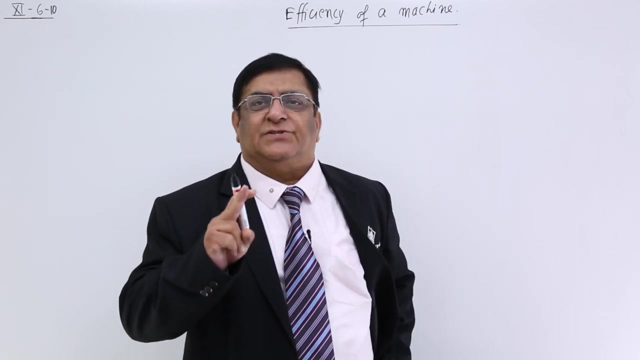 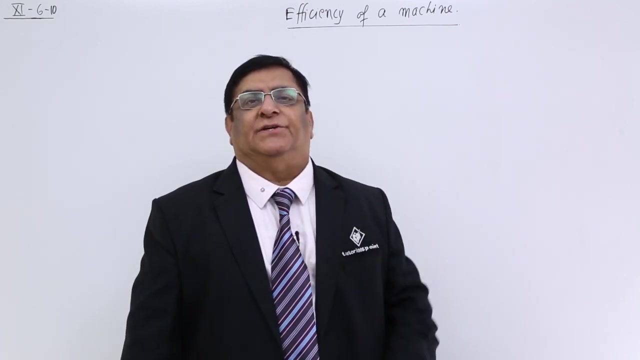 Efficiency of a machine. Efficiency of a machine. What does a machine do? Answer is: the machine is converting one form of energy into other form energy, and that is it is doing the work. Again, what a machine is doing? Machine is doing the work In the work. what happens? One type of energy is being converted to another type of energy. Okay, Then, what is meant by efficiency of the work? 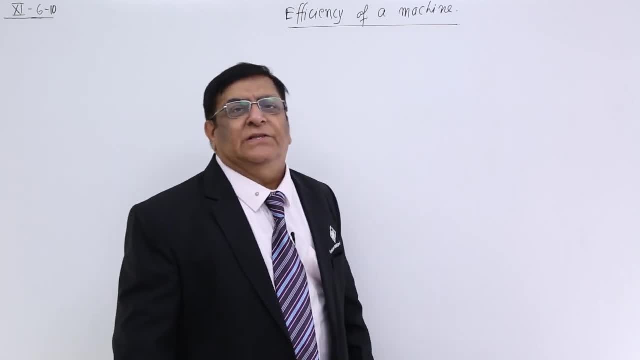 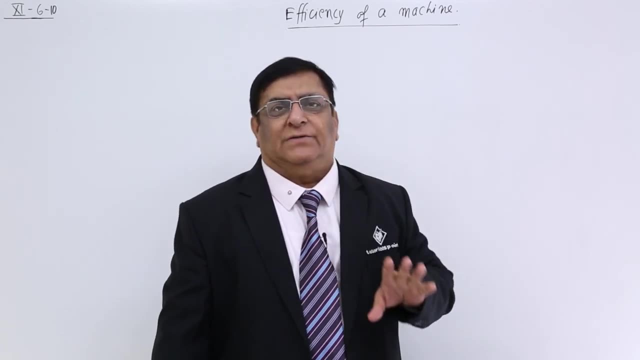 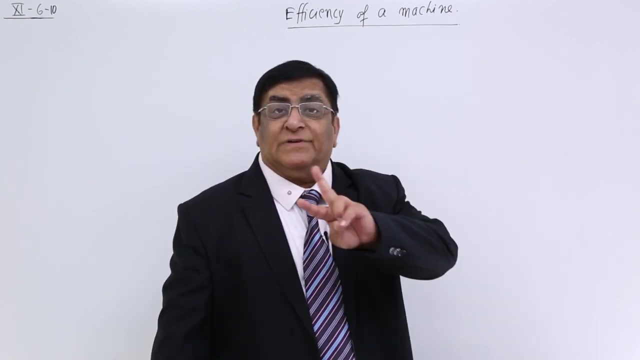 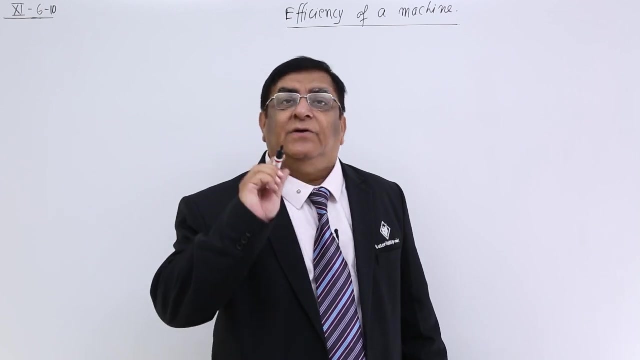 Efficiency of the machine. Now in this we have to understand that work done by a machine per second, that is called power. So whether it is power or work done, it is the same term. Energy is always converted. That means first we give energy to a machine. Machine does not make energy by itself. We give energy to a machine. We will call it input energy. 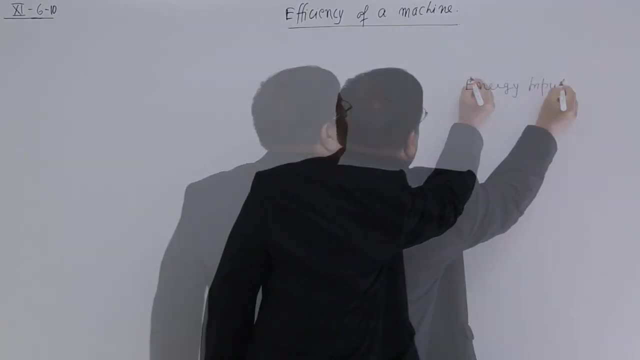 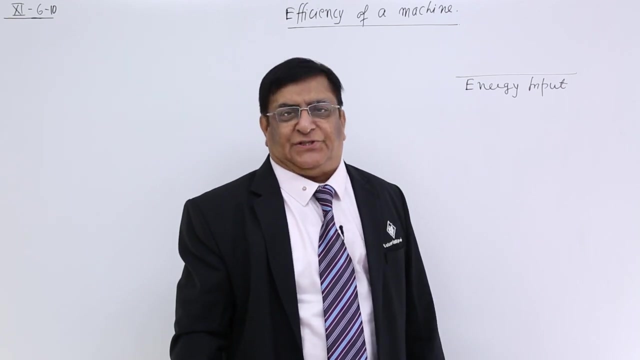 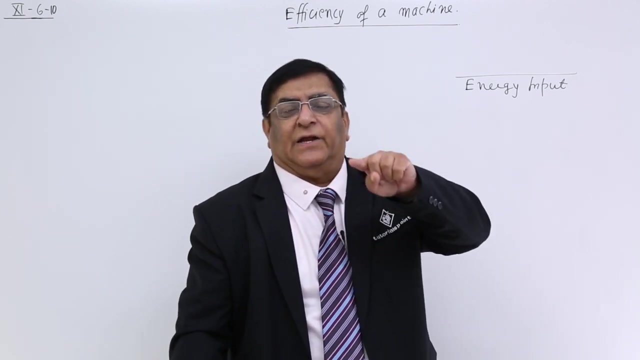 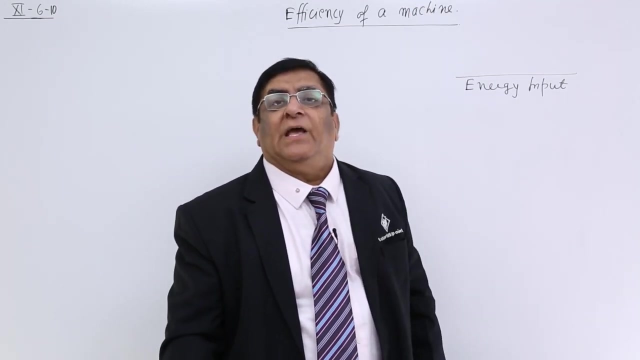 For the machine. it is input energy. Okay, That machine is doing certain work for us. We have designed the machine to give us the work, what we need. If we need a work in which the water has to go up our roof, then the machine is a pump. If we need a machine, if we need work to be done so that heat is taken away, then we have to give energy. 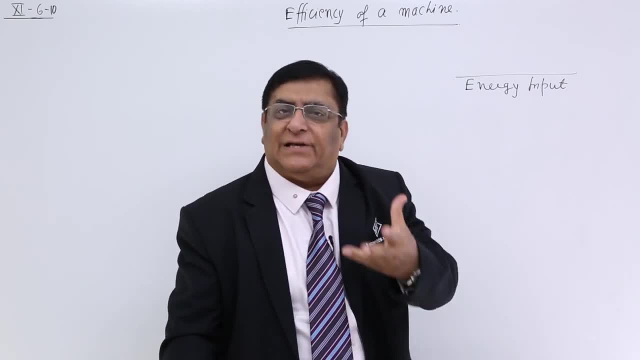 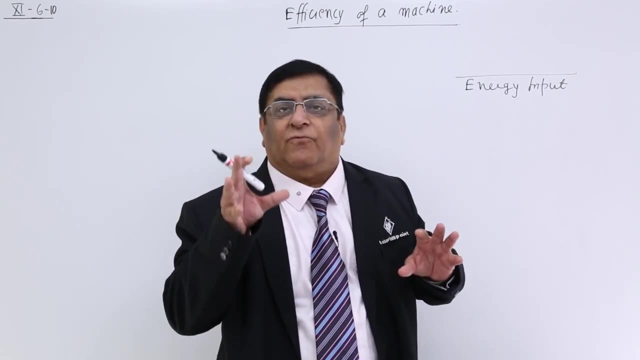 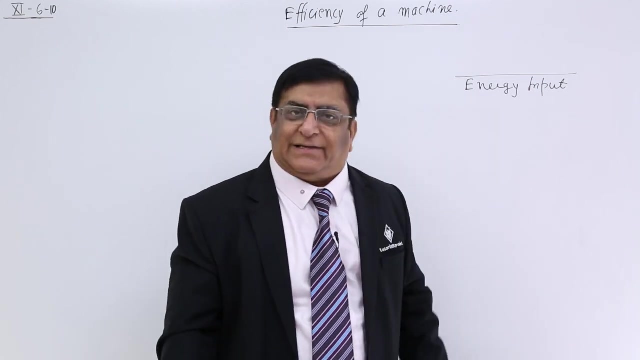 come out from our room, then that machine is air-conditioned. So we design the machine so that when energy is converted from one form to the other form, from electrical to heat, from electrical to mechanical or anything like that, then in between the machine is. 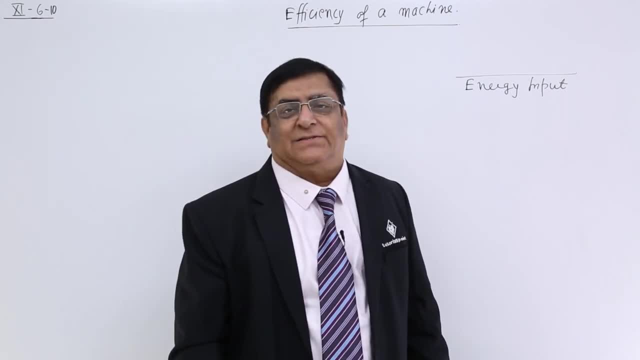 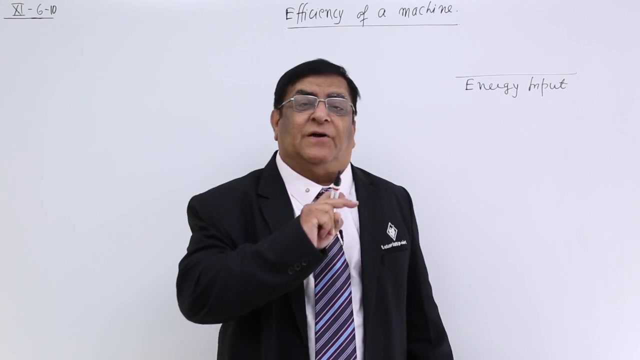 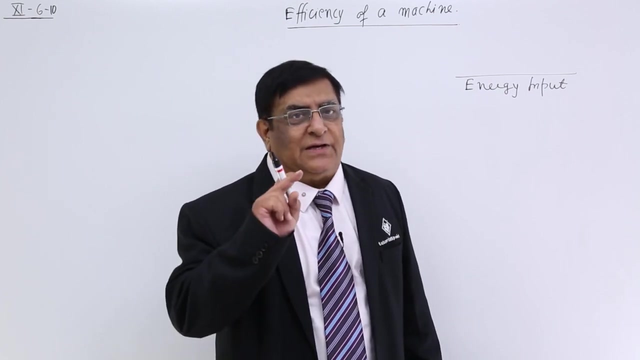 doing work for us. Yes, that is what happens. There is no lost of energy. that means their energy does not destroy it. Energy is only converted. but in the process of conversion, what is done? We call it work done. So we give electrical energy to a pump That pump. 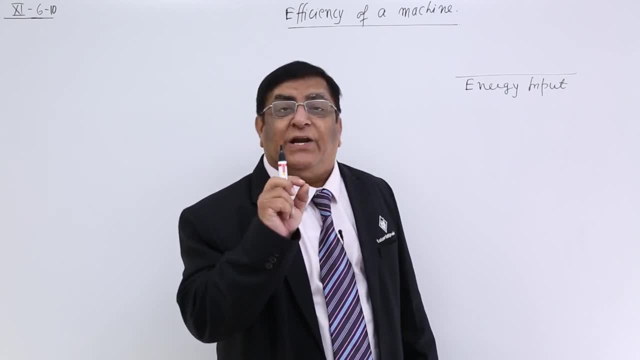 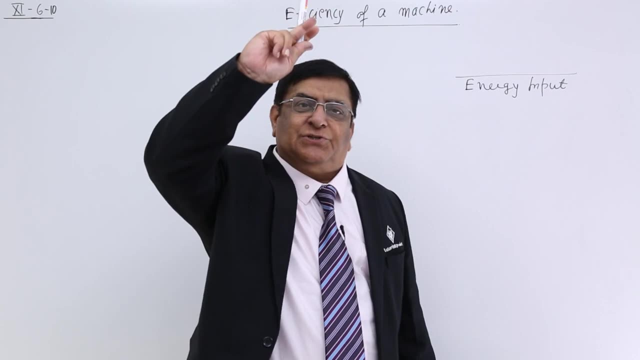 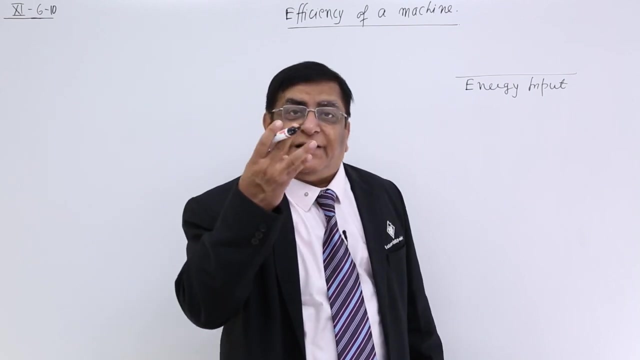 converts that electrical energy. So we give electrical energy to potential energy of the water by rising it to height h and giving it an energy mgh. So there is a conversion of energy. but in this conversion of energy the work done. that is what we wanted pump to do. So we say our work is. 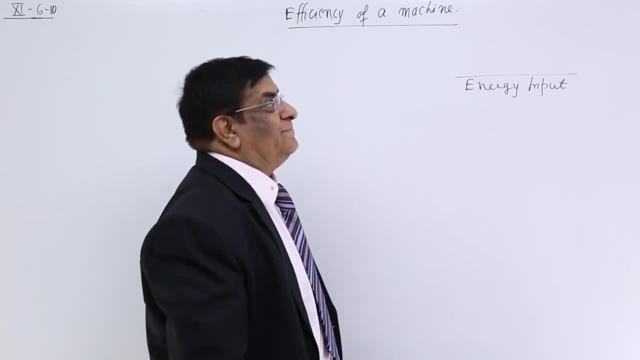 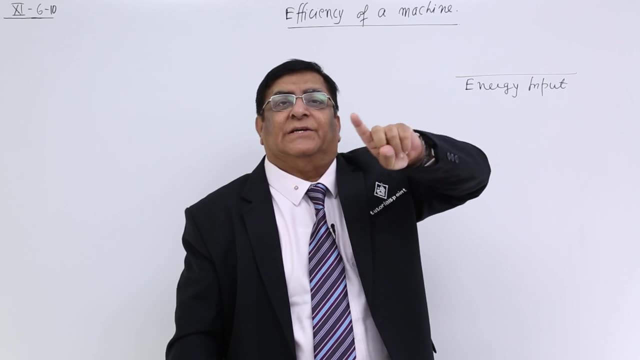 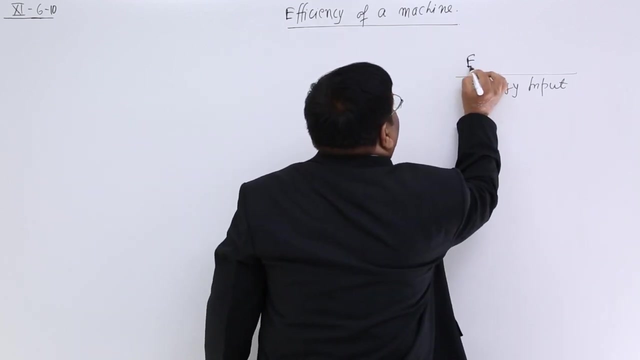 done. That is work done. So when the pump raise the water up, we calculate how much work it will do. So that is our work done. So when the pump raise the water up, we calculate it is doing. whatever work pump is doing, we will call it energy output. so what is this? 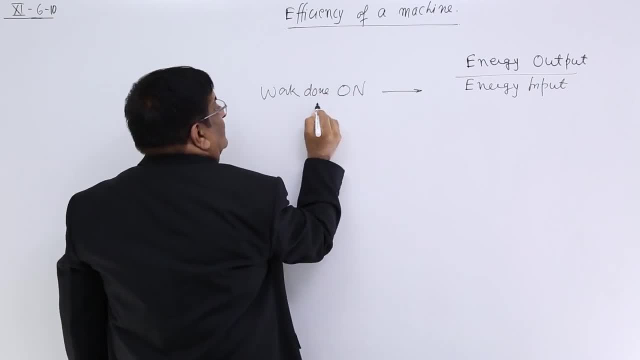 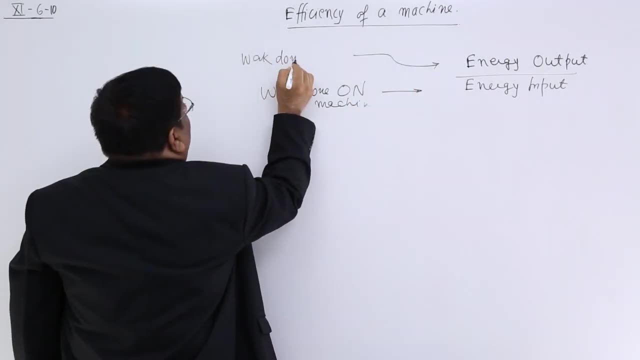 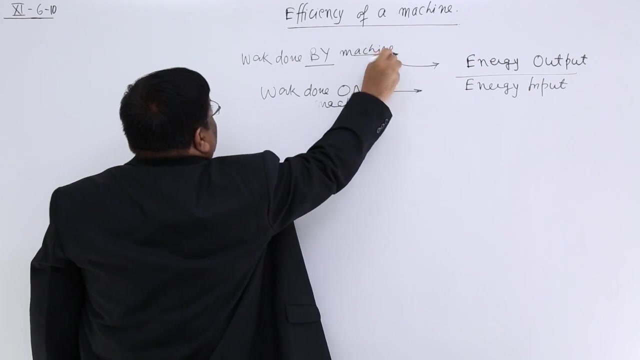 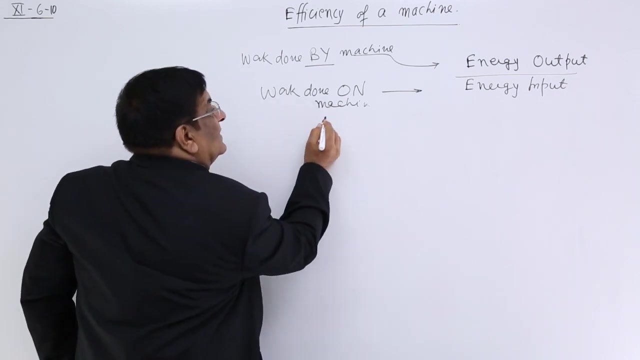 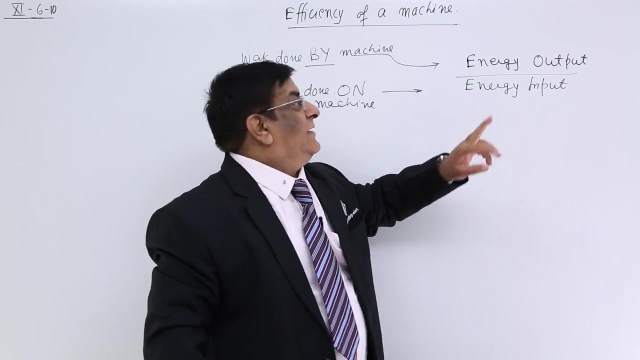 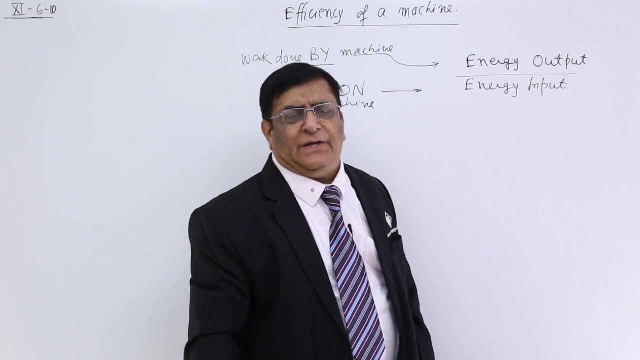 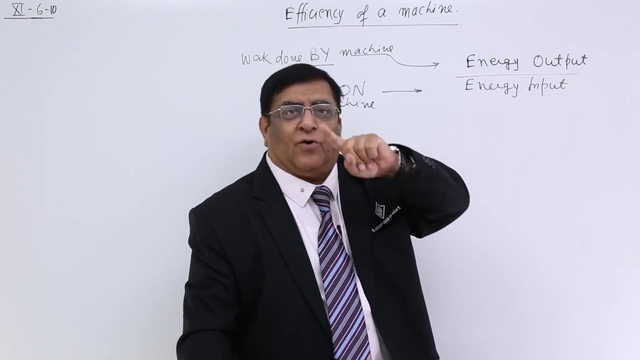 work done on machine. and what is this work done by machine? so this is work done by machine- is energy output. work done on machine is energy input and we have found that these two energies are not equal. why these are not equal- by conservation they should be equal. answer is: whatever energy we give it as input, it is not necessary that. 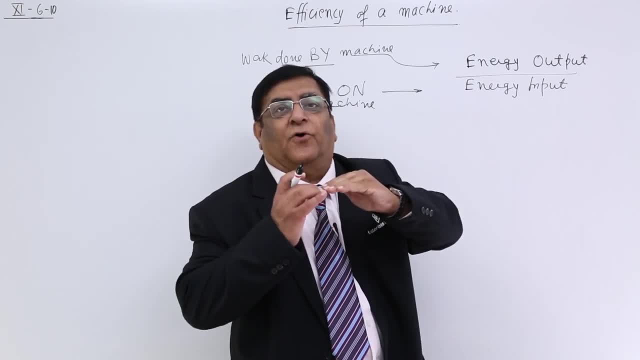 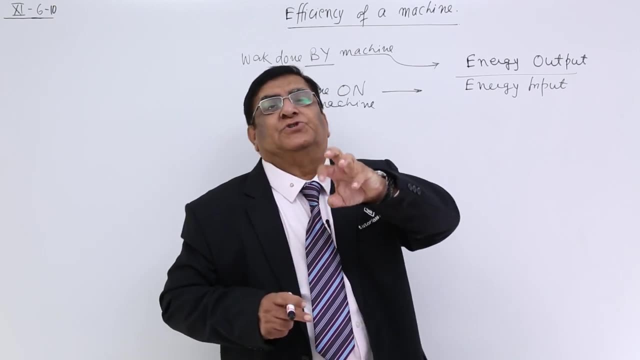 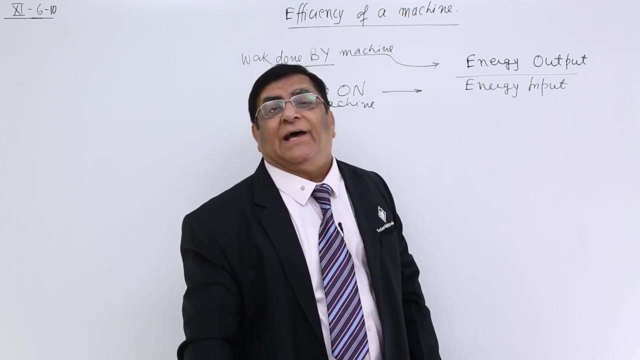 all the energy is transformed. 215.etz. the form we want, what i want: all the energy i give to pump. i wanted that all energy should be transferred as potential energy of water so that water goes up to the pump. but what happens? the pump is doing certain work, it has got certain friction, it has got a motor. 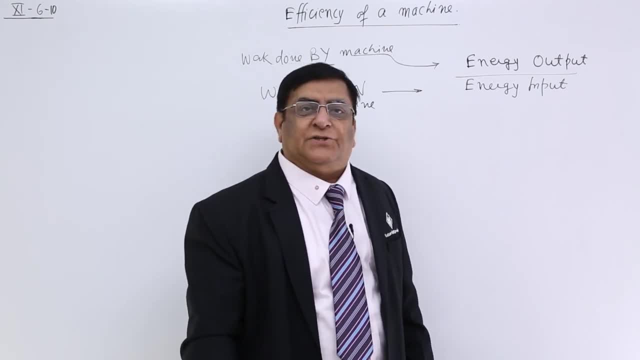 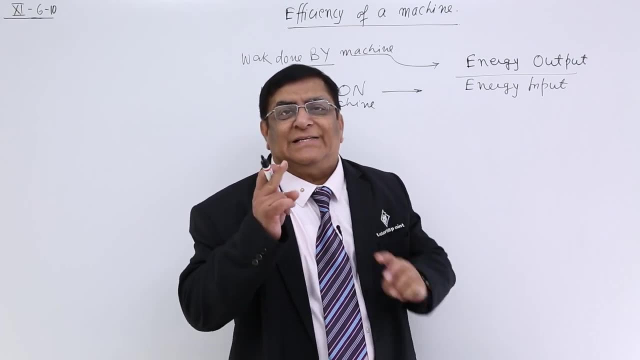 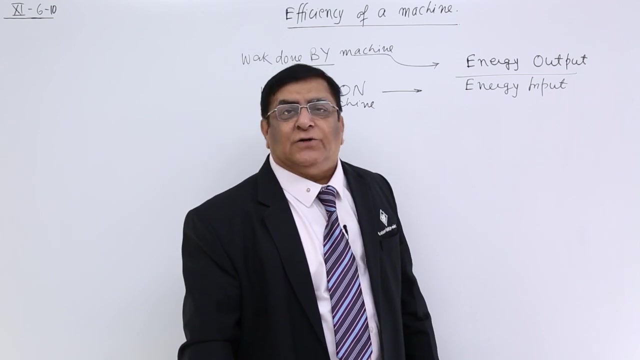 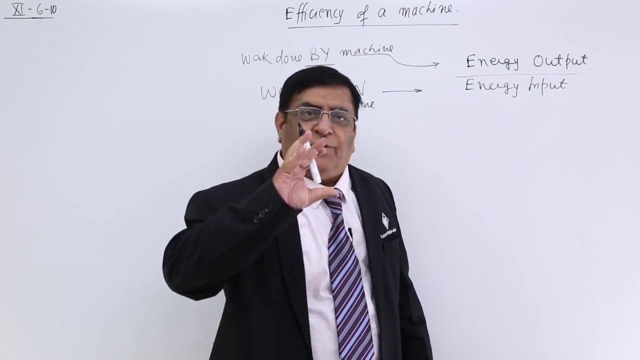 that motor gets heated up due to friction and due to heat radiation from the motor coils. so that is the energy required for the pump to operate itself and that is the loss of energy. loss means it is not destroyed, it is converted to work, it is converted to a format. 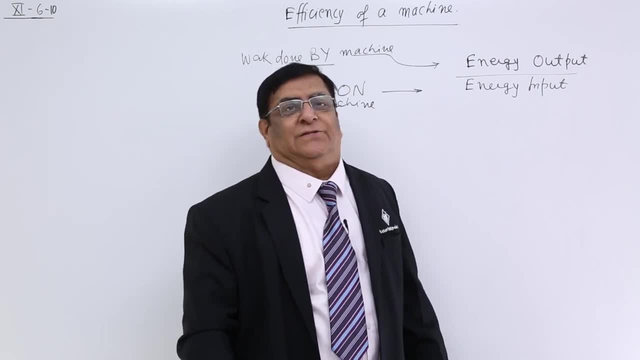 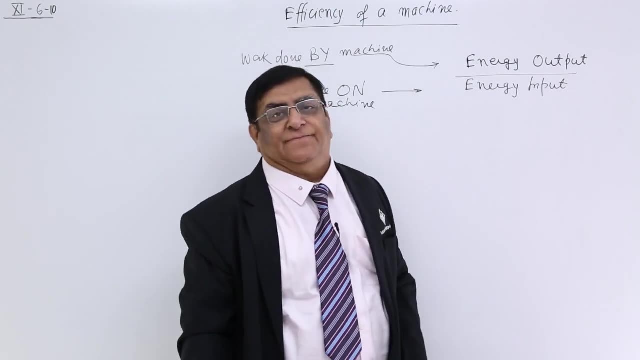 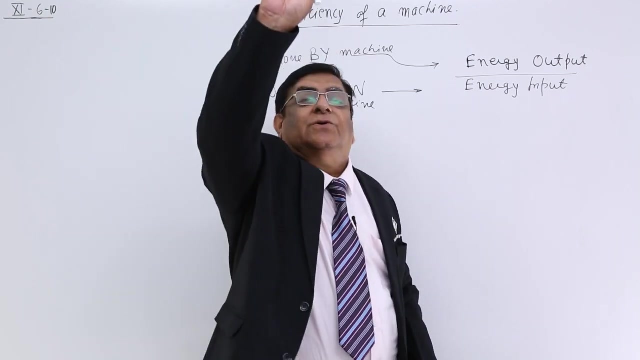 which i do not want. so i am using the word loss. loss converted to heat, that heat of the motor. the motor gets heated up that is radiated out in the nature. So for me it is a loss because I gave energy to the pump so that it is converted to mgh. 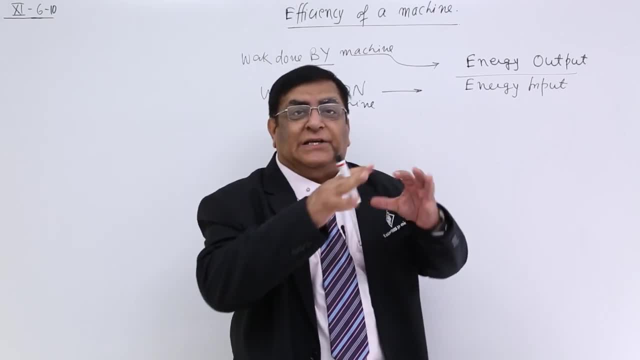 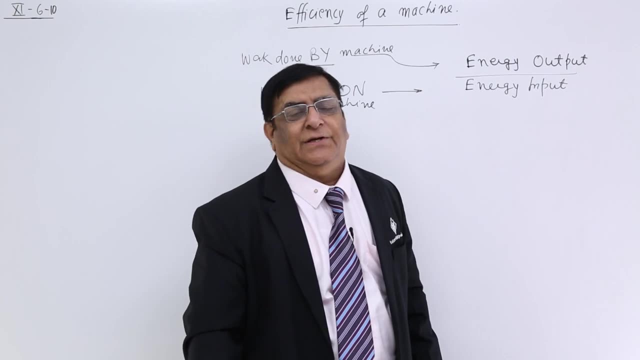 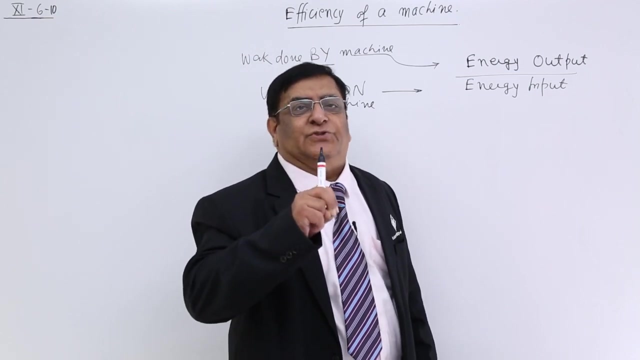 of the water, But some of the energy it has used in the heating itself and to radiate out that heat. For me it is a loss, but it is energy converted to heat. it is not destroyed from the nature. I am concerned with that energy which is used for lifting the water up, and that is energy. 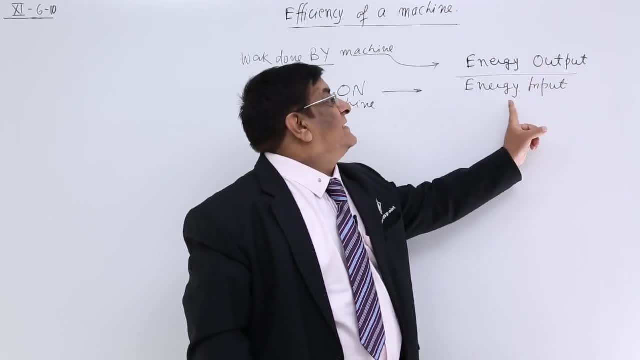 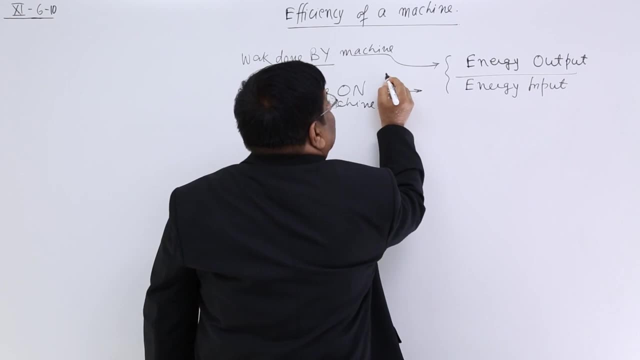 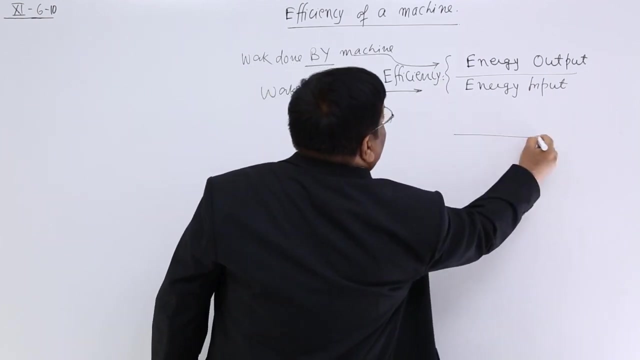 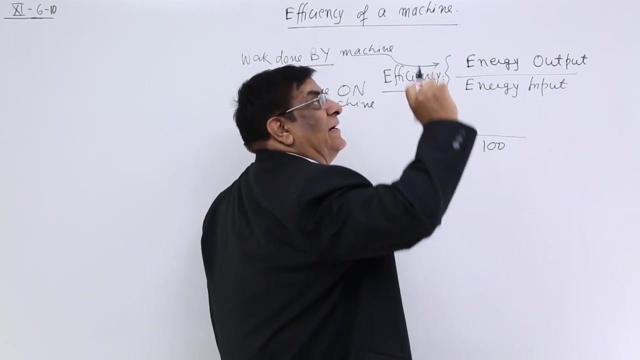 output. So this energy output is always less than energy input And this shows me this ratio. I call it efficiency. Suppose I give energy input 100 to a machine And it lifts the water up, I calculate how much work it is doing and it is doing a work of 60 joule per second. 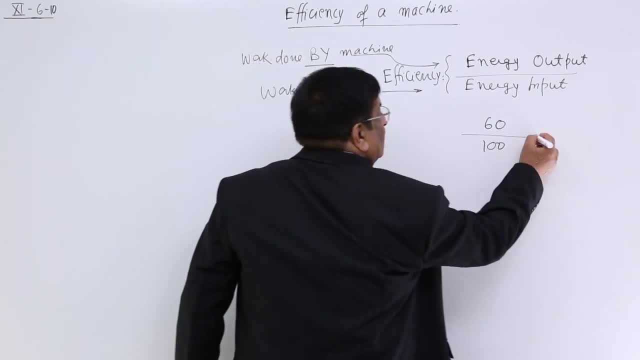 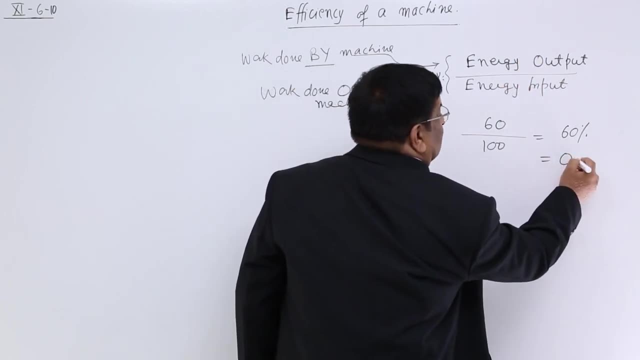 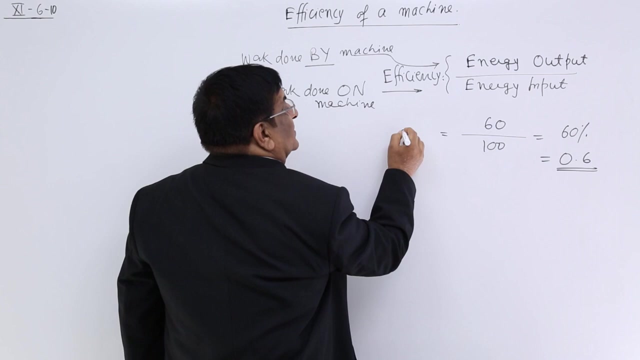 I am giving it 100 joule per second. So I say that my machine is 60% efficient, or my machine's efficiency is 0.6.. This is efficiency of my machine and I will use the letter eta, Eta, Eta. 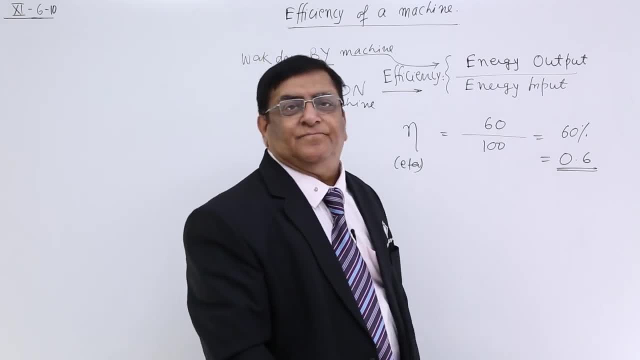 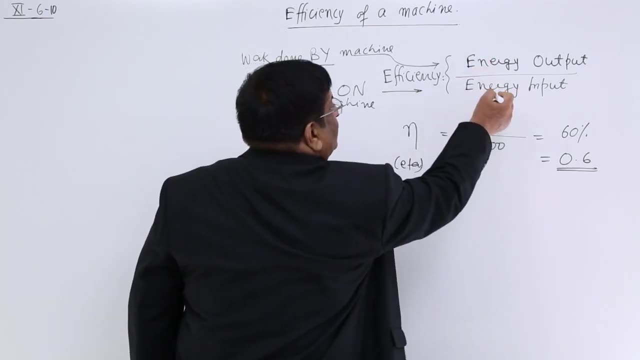 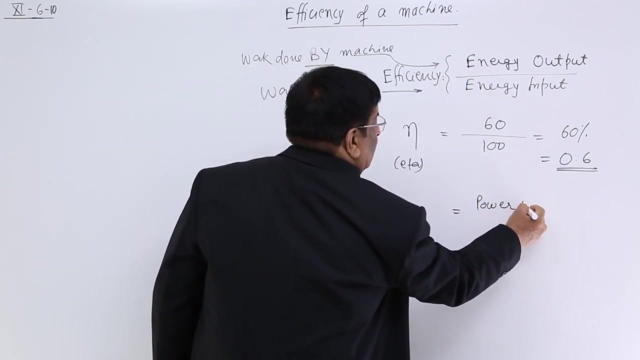 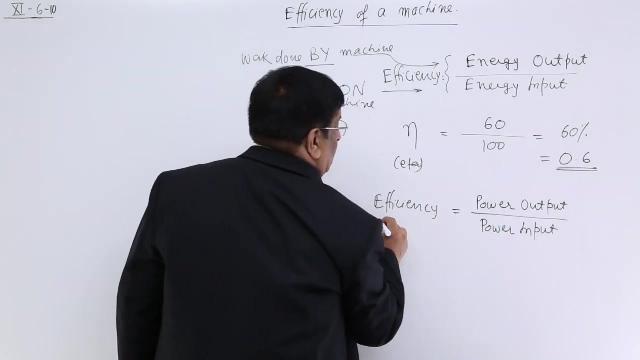 Eta. Eta For efficiency 0.6.. So this is efficiency. So now this you have to remember: energy per second is the power. So we can say power output divided by power input is efficiency of the machine. So please remember this formula. 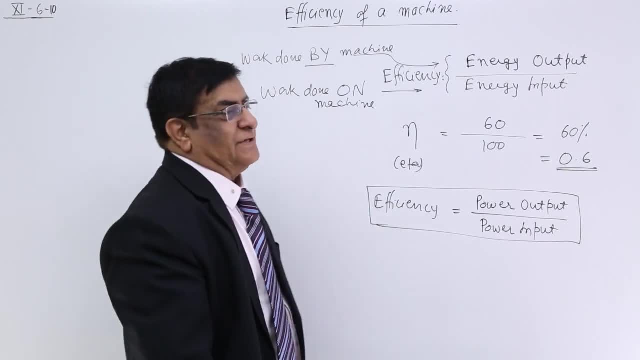 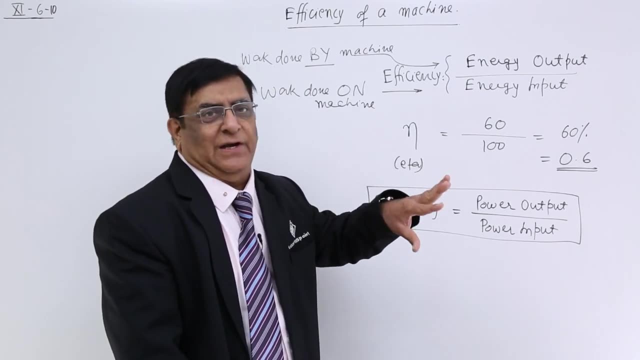 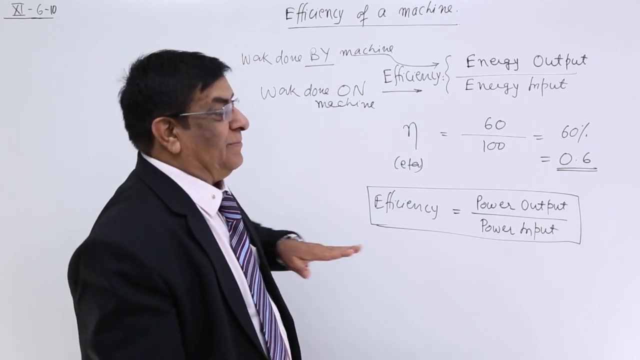 Power output divided by power output. Power output, Power output input is efficiency of the machine. with this, power input is what it may be, another format. we are giving it power in electrical form. power output may be in any form: it may be heat, it may be mechanical energy, it may be kinetic. 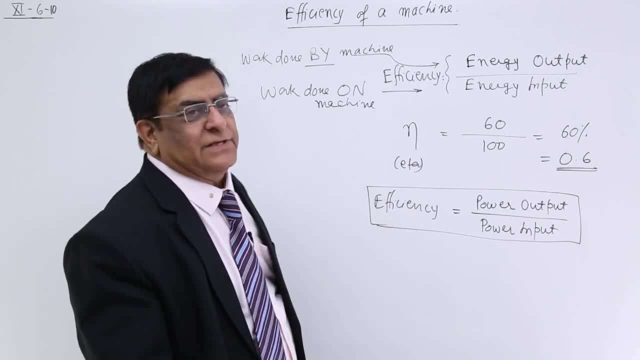 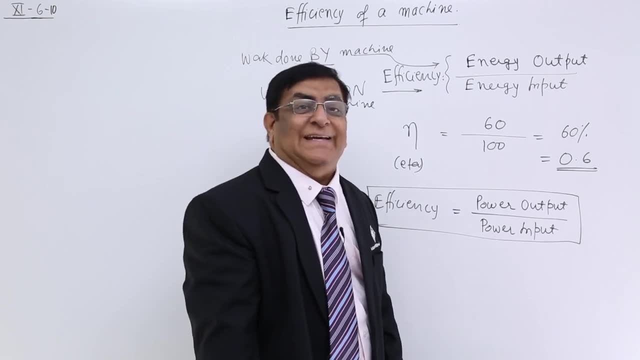 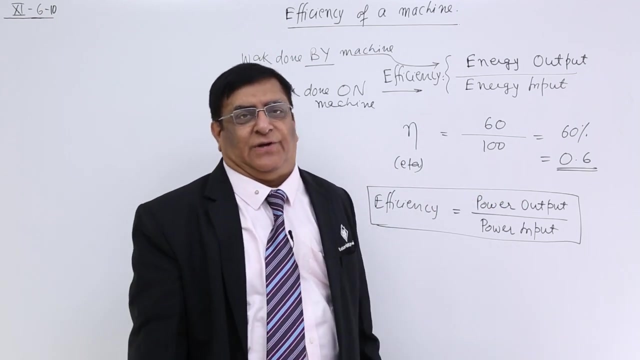 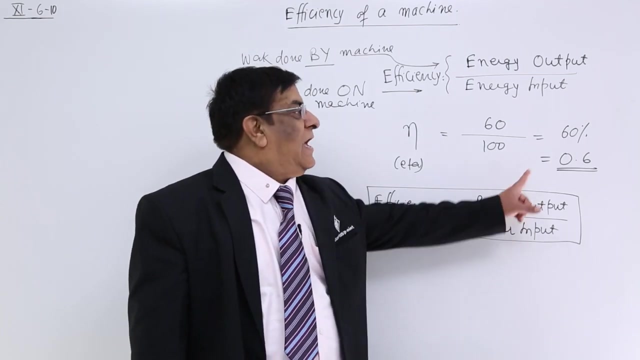 energy, anything, and that shows the efficiency. so any machine in the nature is never 100% efficient because it needs some energy to be radiated out. that we will study in the topic of thermodynamics. but the thumb rule: we remember that no machine in this universe is having efficiency equal to.